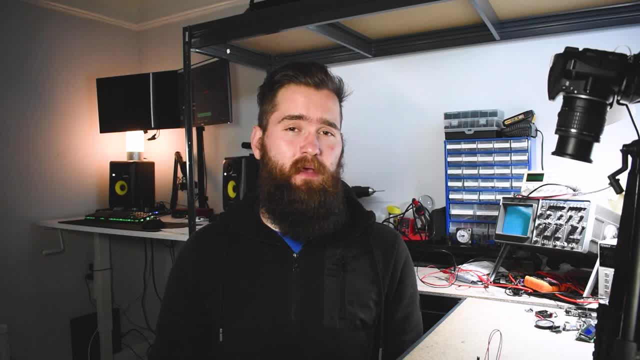 that make up a microcontroller: CPU, memory and IO or input output to connect to our external peripherals. The interesting thing about microcontrollers is that they actually have all three of those components all built into a single chip. This makes them extremely useful for smaller devices that. 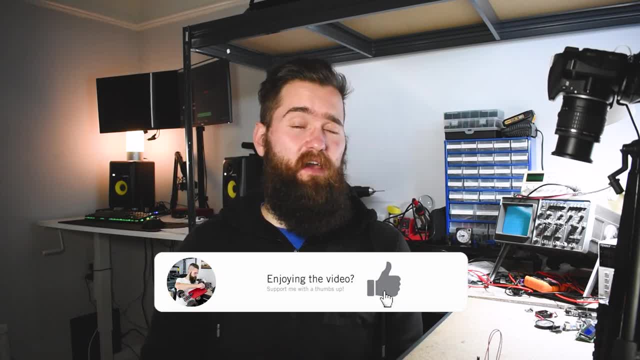 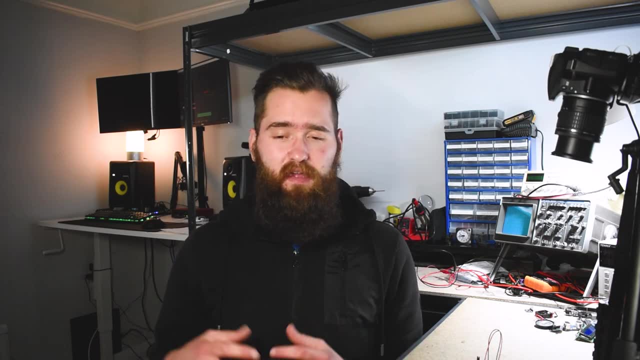 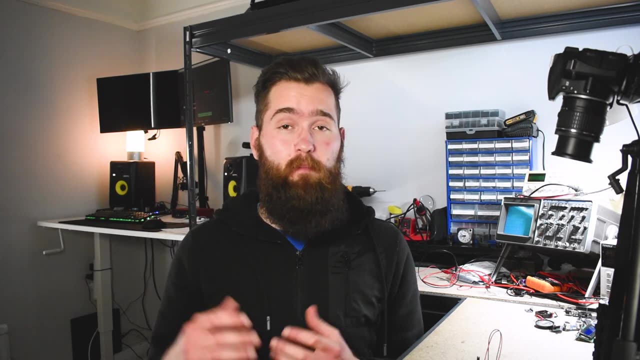 we tend to call embedded systems. You've probably already heard of IoT or Internet of Things, and that whole idea basically stems from these kind of devices. The idea behind IoT is to have all these individual devices all connected together and communicating. So what classifies as an embedded system? 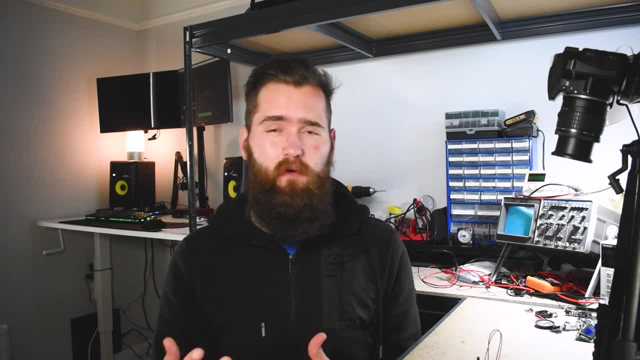 Embedded systems are all around us, And it's funny because in the world today, we tend to take everything for granted. Something like this TV remote, for example. Most people are just going to grab it, use it and not really think too much about what's going on inside. 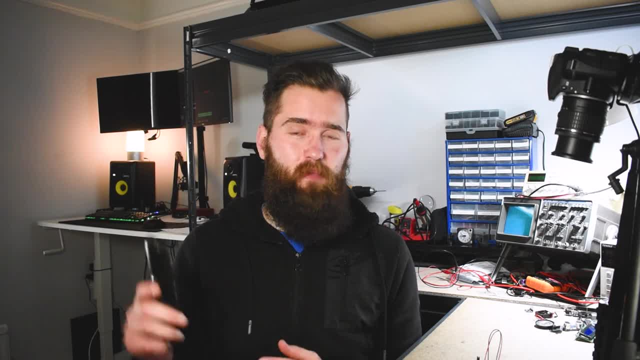 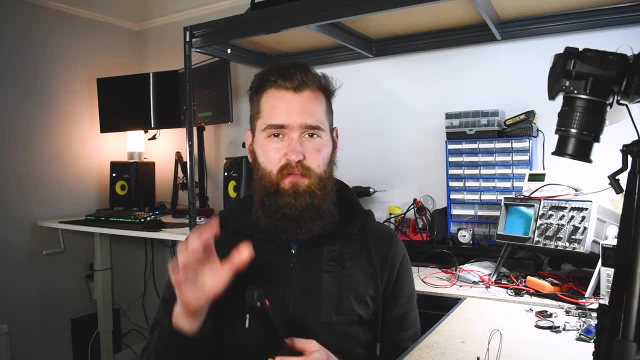 But a lot of effort goes into something even as simple as this, And that's what I love about electronics and embedded systems. There's kind of like this whole other world going on underneath what we see at face value When you dive into it and start asking all these questions about how things like this work. 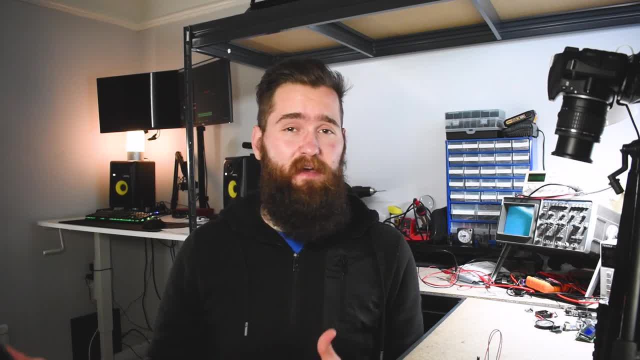 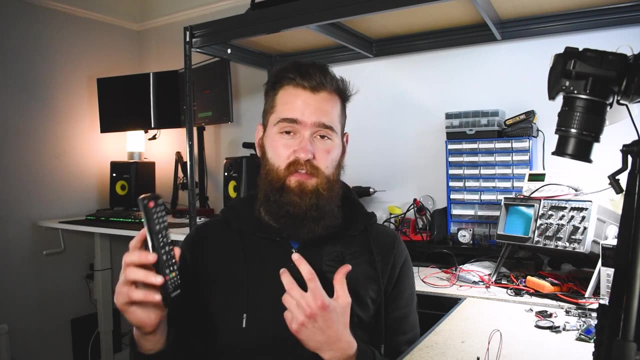 you start to become a lot more grateful for all the technology we have today that makes our lives so much easier. So an embedded system is a digital device that is dedicated to a specific task. So, for example, this TV remote is an embedded system. It has only one job to do, which is to send. 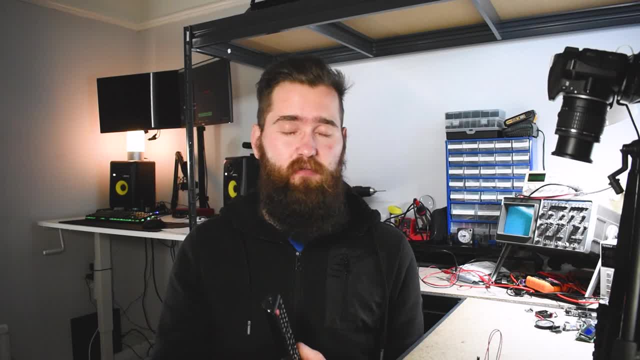 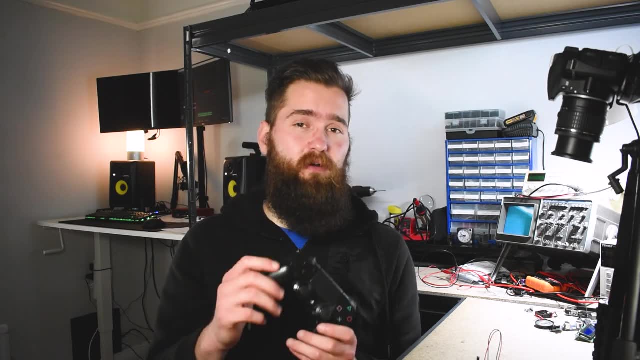 frequencies to the TV so that you can control and use it. This PS4 controller is also an embedded system. It also only has one job to do, which is to send your user input data to the PS4 via Bluetooth. An example of something that isn't an embedded system would be your smartphone or 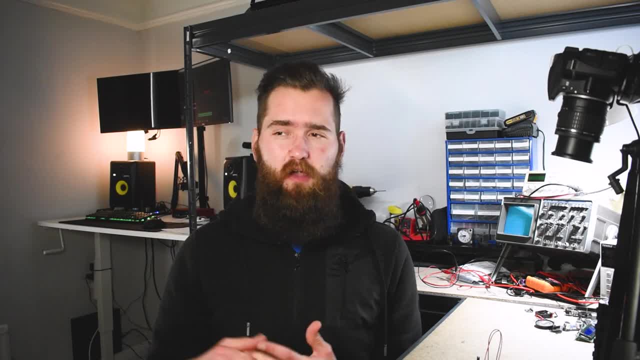 desktop computer. Smartphones and desktop computers run on complex operating systems that are generally designed to multitask. Your smartphone, for example, can be whatever you want it to be. You can play games on it, you can phone people, you can text people, you can use. 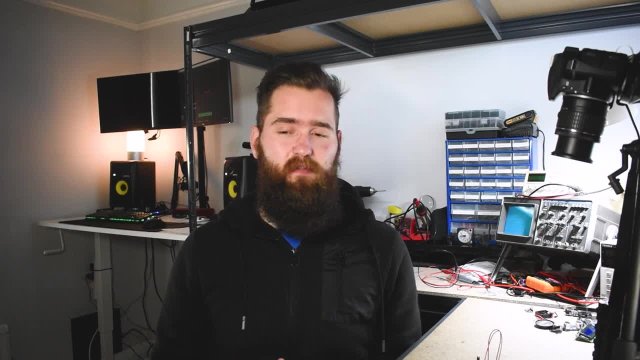 the camera. you can browse the internet. It has so many different uses That is not considered an embedded system. Other examples of an embedded system would include digital watches, microwave ovens, washing machines, and the list just goes on and on. 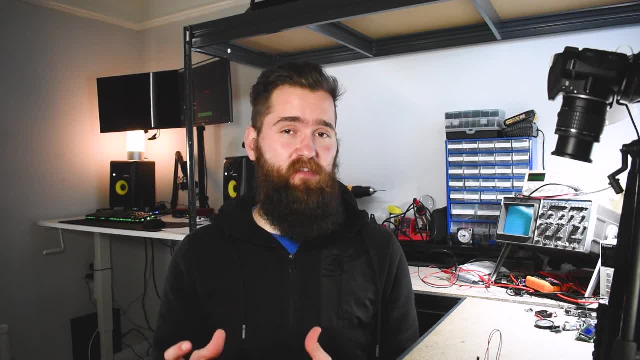 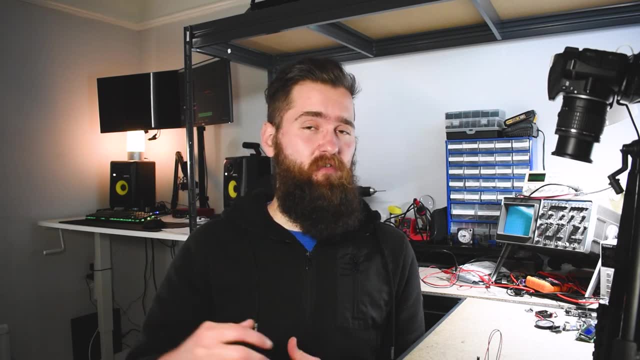 The important thing to remember, though, is that at the core of all these devices is a microcontroller, just like the ones we're looking at here. A microcontroller on its own isn't very useful, So let's talk a little bit about peripherals. What classifies as a peripheral? 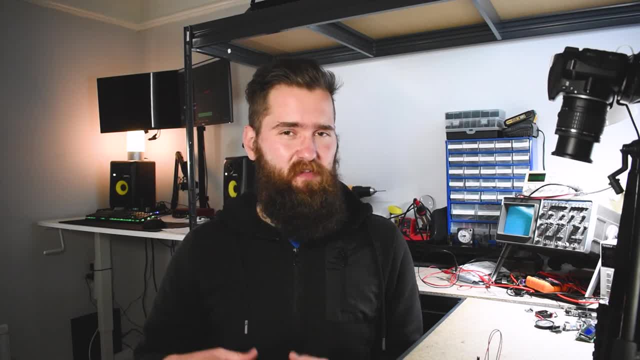 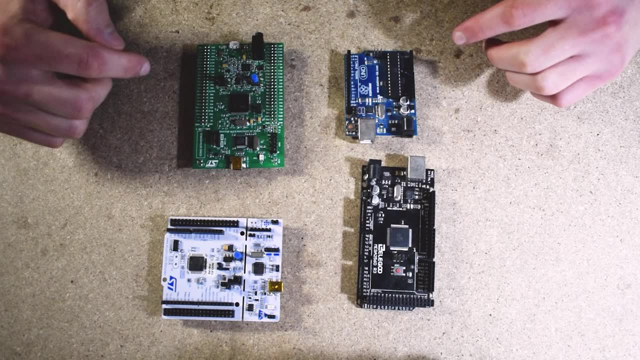 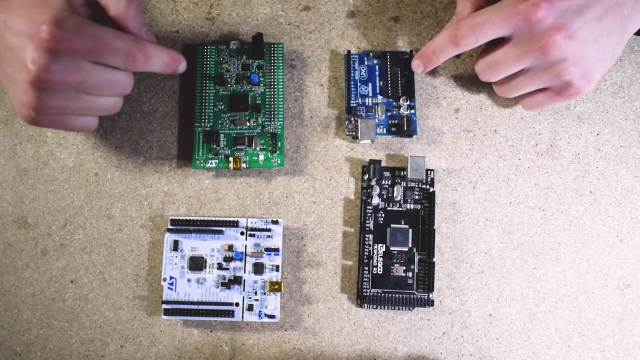 A peripheral is any electronic device or component that's external to the microcontroller. Notice, on these development boards we have a lot of other components and ports around the outside of the chip. These ports and components all connect to the tiny pins on the chips And we can use these ports around the outside to connect our 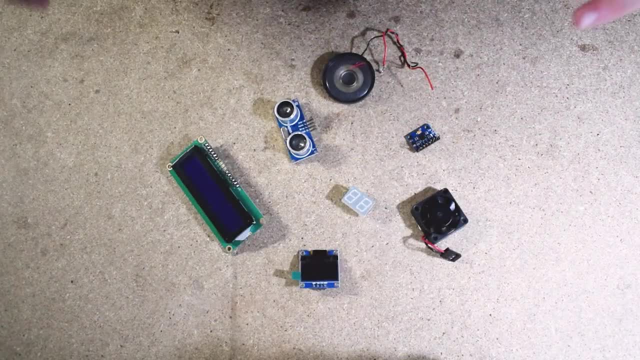 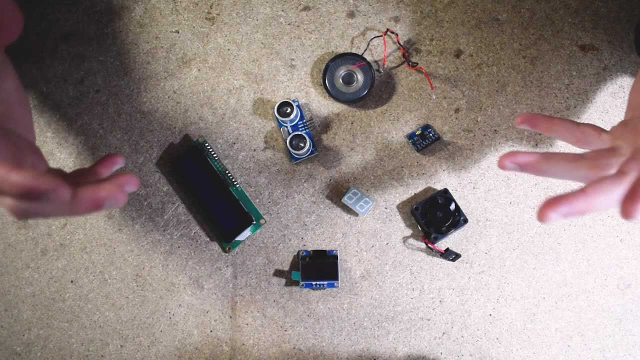 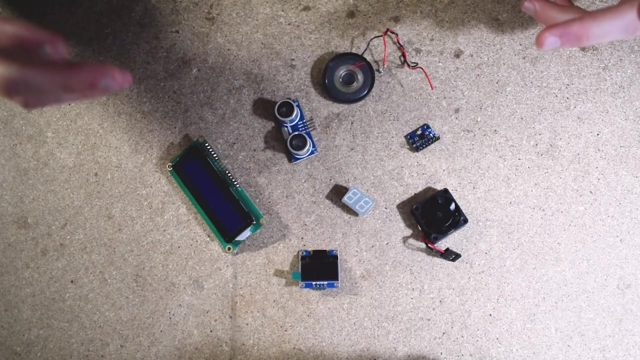 microcontroller to external devices and peripherals. I have a few devices here that will be considered as peripherals. The simpler peripherals are things such as keypads, LEDs, microphones, buzzers, and again, the list keeps going. But then you can have more advanced peripherals such as integrated circuits, sensors or LCD displays. 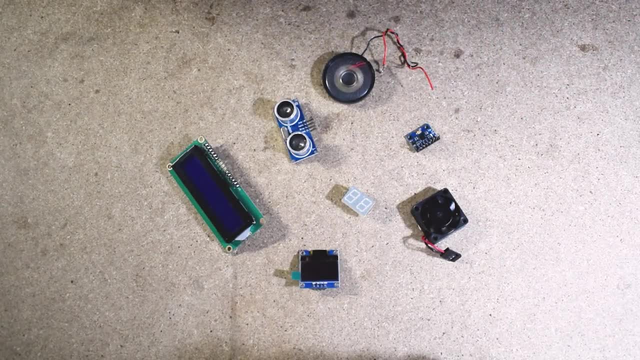 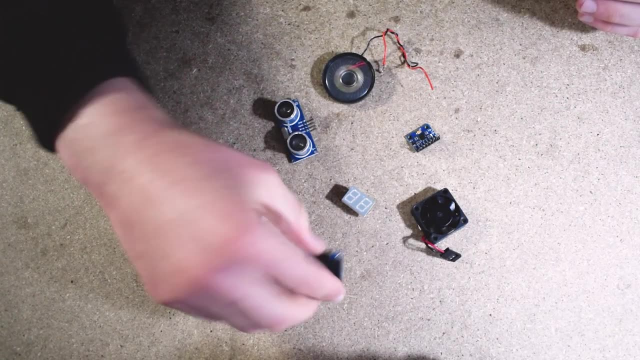 These type of peripherals will use communication protocols such as I2C or SPI, But that's a topic for another video. You can see here we've got two LCD displays, both different sizes. We've got sensors. This is an accelerometer gyroscope. 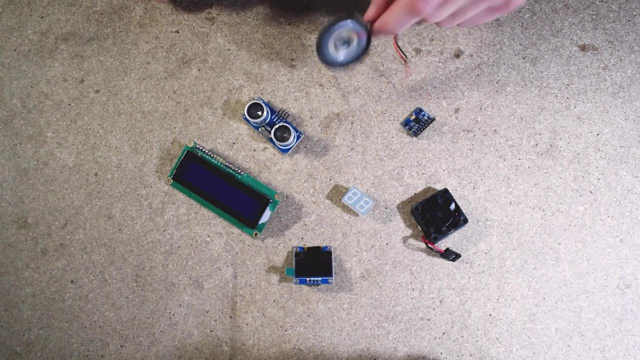 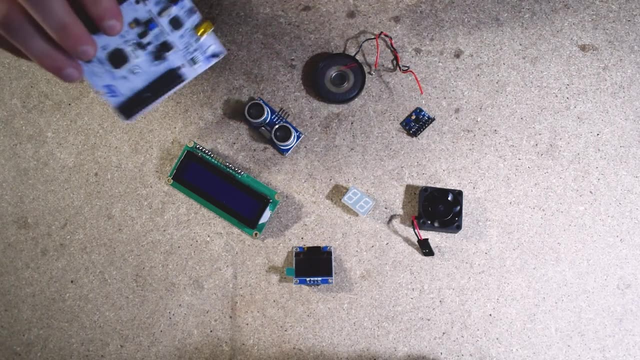 This is an ultrasonic sensor, This is a speaker And obviously this is a tiny little 5 volt fan. All of these are classed as peripherals Because they're external to our microcontroller And we can use our microcontroller to control and talk to all these different devices. 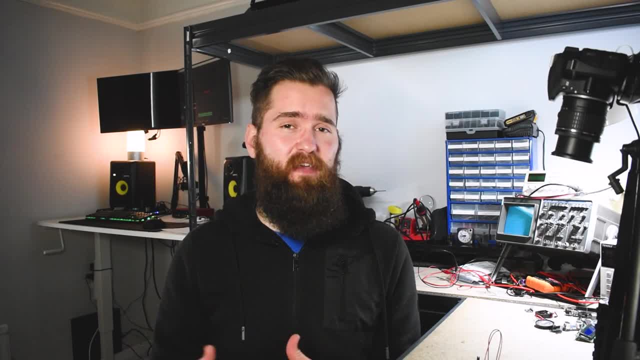 These kinds of boards that we're looking at here are designed for testing and development purposes. If, for example, you wanted to develop your own alarm clock, you would first build and test the system on one of these boards before you go ahead and create a custom printed circuit board. 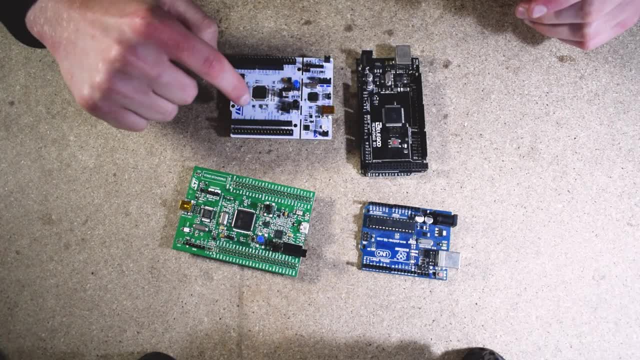 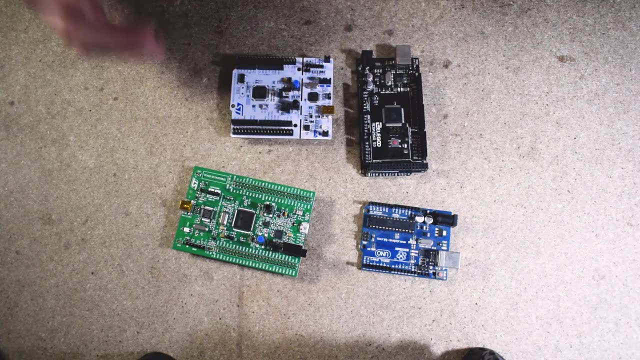 These boards are generally quite big, but you actually only need the chip and a few other components to run an embedded system. The manufacturers generally add in a few more components for you so that you can experiment and play around with stuff that already exists on the board. 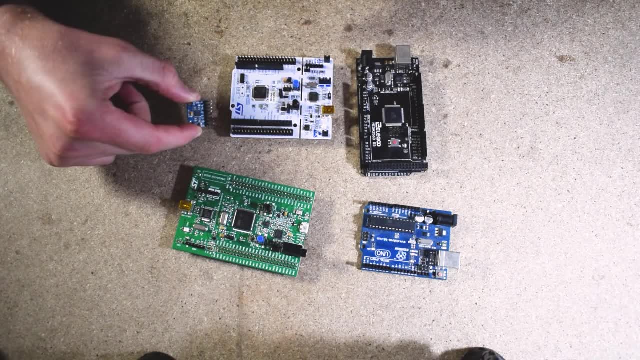 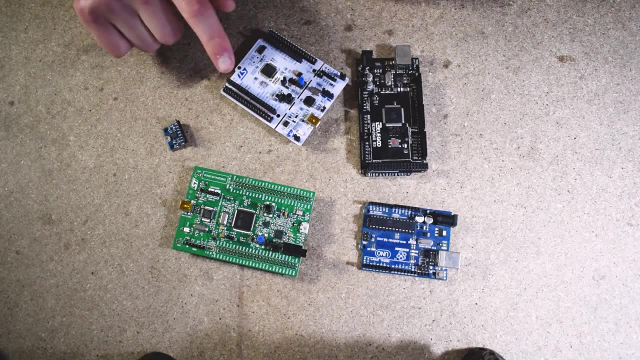 For example, if we wanted to interface to this accelerometer and gyroscope, we would have to connect all these pins up to some of our external pins on the board, And then we could use a communication protocol called I2C to communicate with this other device and fetch information from it. 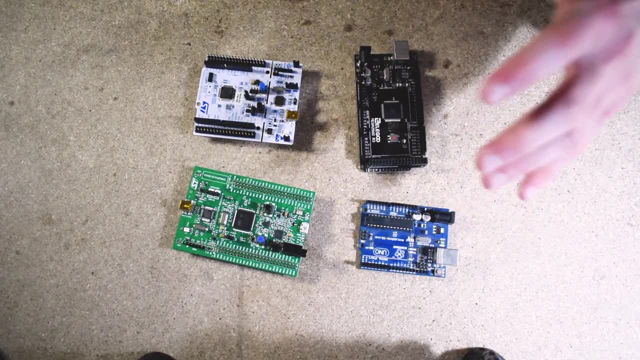 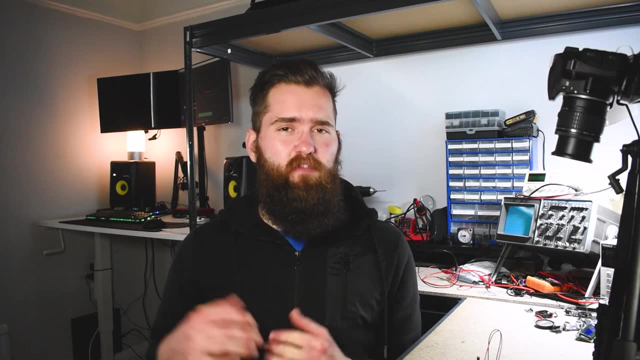 These two boards here are Arduino boards and they both contain AT mega microcontrollers. This is a great way to use Arduino as a real hardware development platform. The software tools are very limited and, honestly, the boards are aimed at kids or hobbyists who are just looking to learn and play around with really basic electronics. 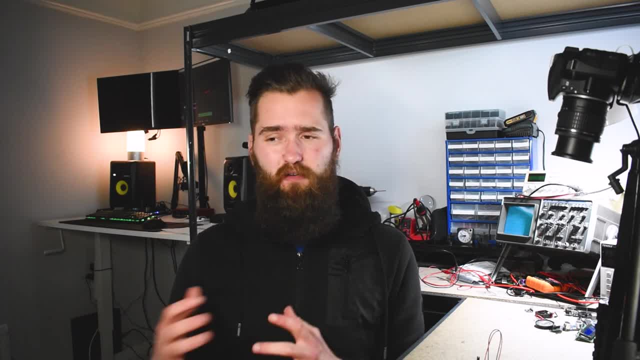 They're great boards if you want to prototype something super fast, but from my experience in industry, if you're serious about learning hardware development, you'll want to stay away from Arduino and go with something that's a little more capable and just more respected in the industry. 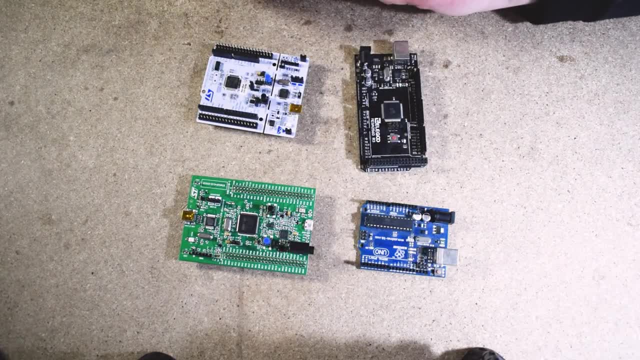 These two boards here were created by ST Microelectronics. These two boards here were created by ST Microelectronics, One of the most reputable semiconductor manufacturers in the world. One of the most reputable semiconductor manufacturers in the world. Both boards have ARM Cortex-M4 microcontrollers that are industry standard and packed full of extremely useful features. 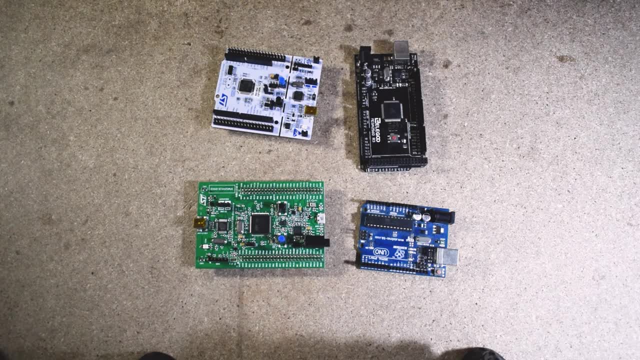 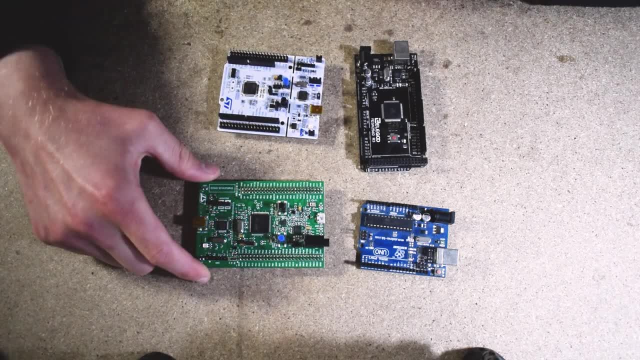 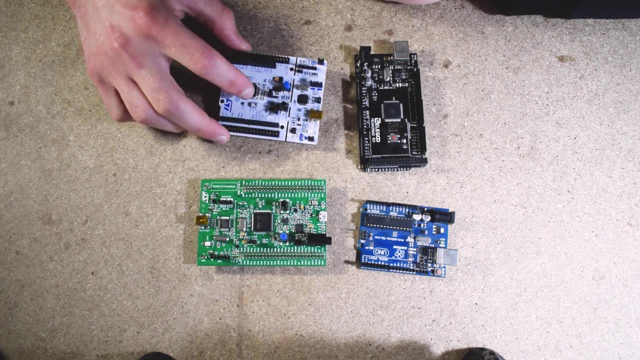 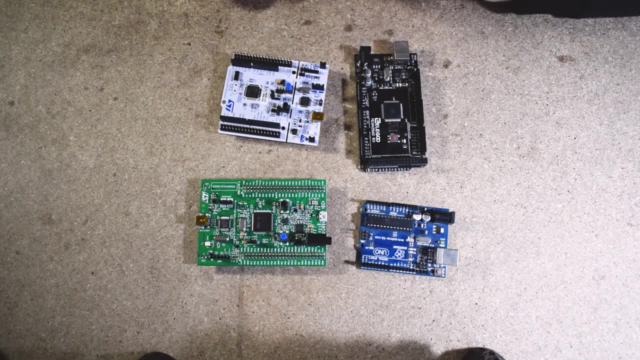 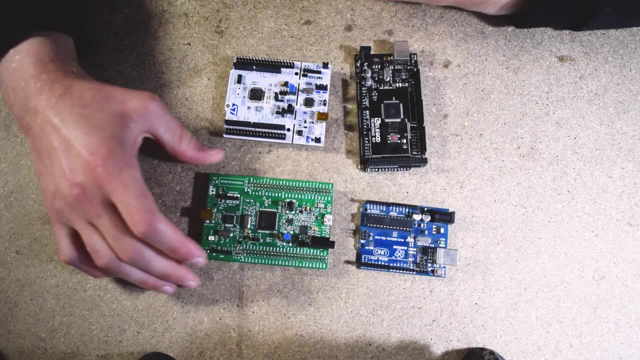 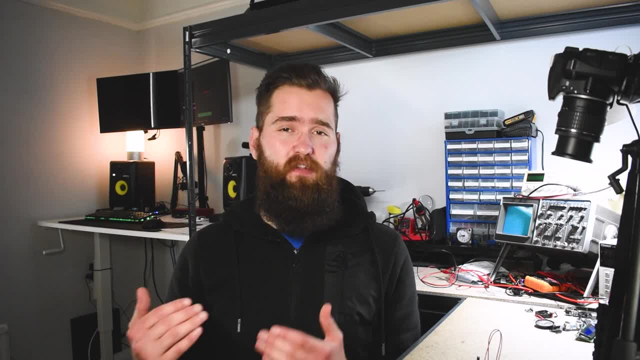 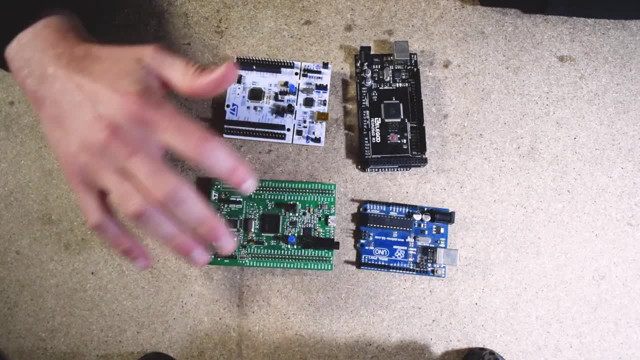 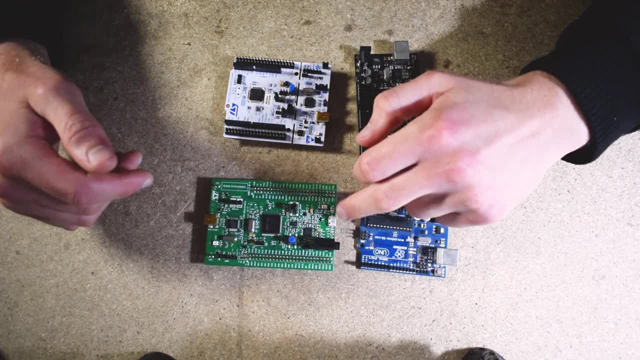 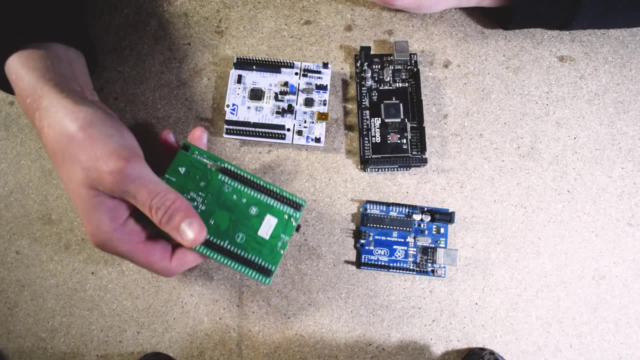 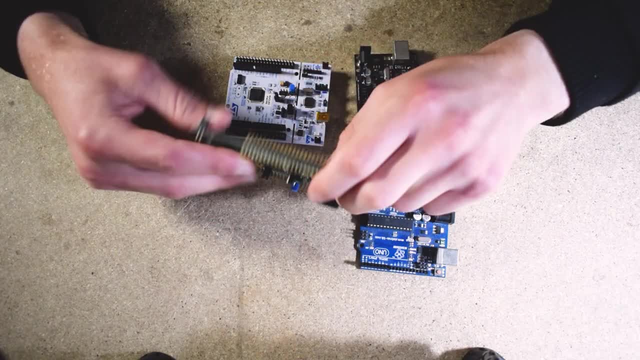 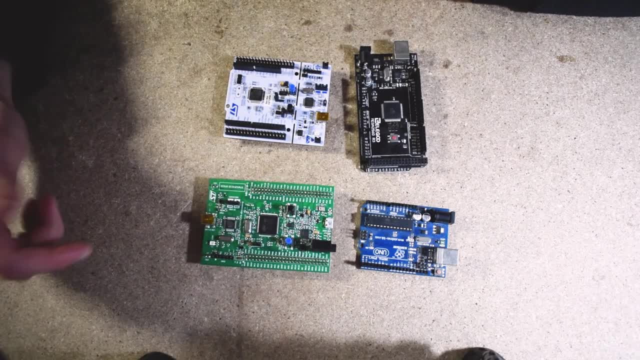 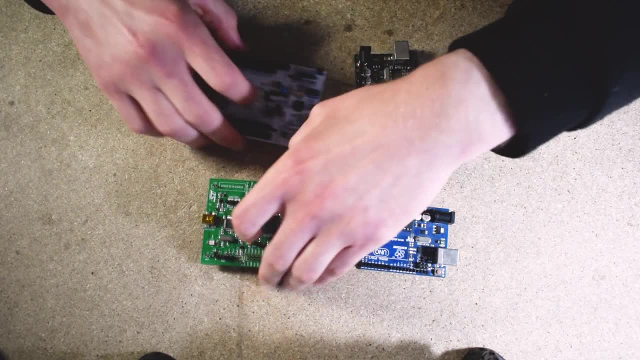 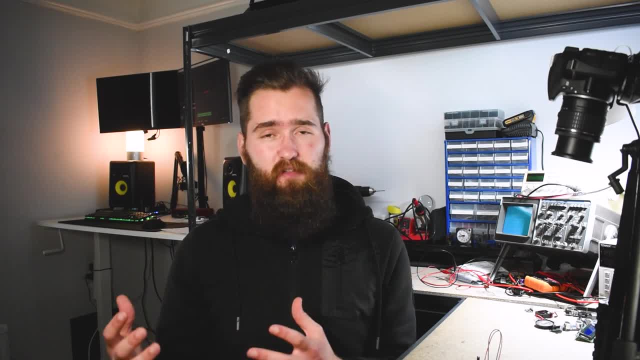 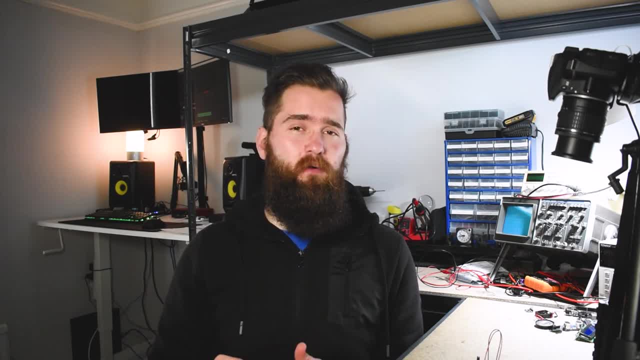 This nuclear board has a smaller 64-pin chip, whereas the F4 Discovery board has a larger 100-pin chip. This nuclear board has a larger 100-pin chip, whereas the F4 Discovery board has a larger 100-pin chip. This nuclear board has a larger 100-pin chip, whereas the F4 Discovery board has a larger 100-pin chip. 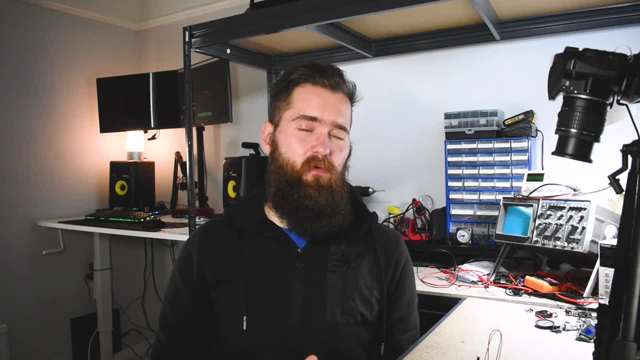 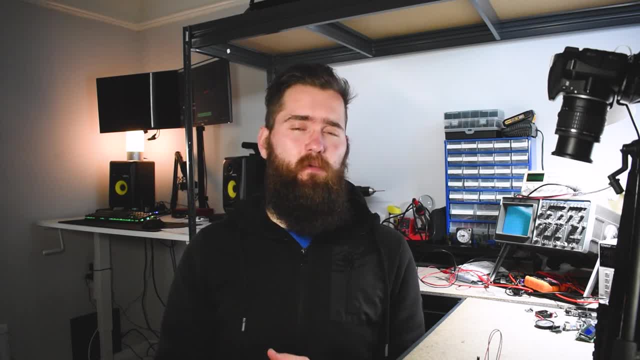 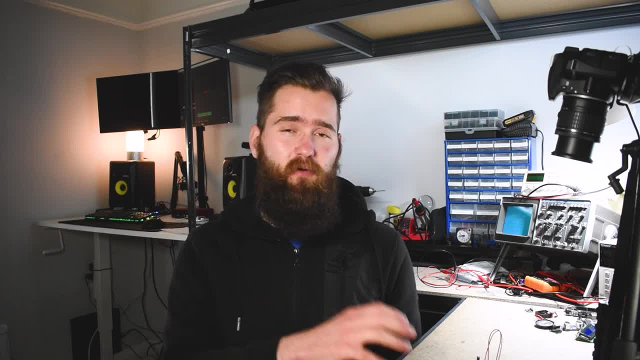 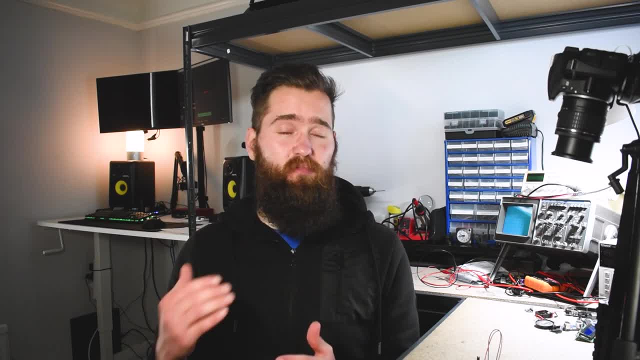 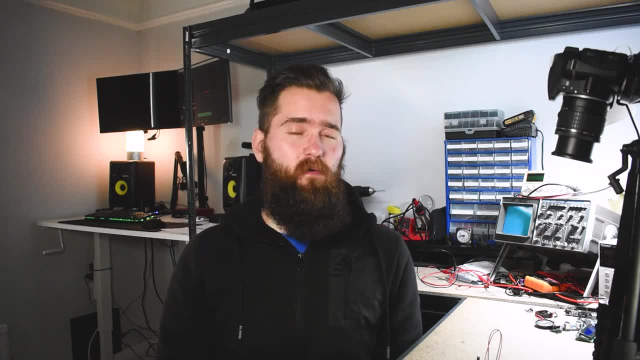 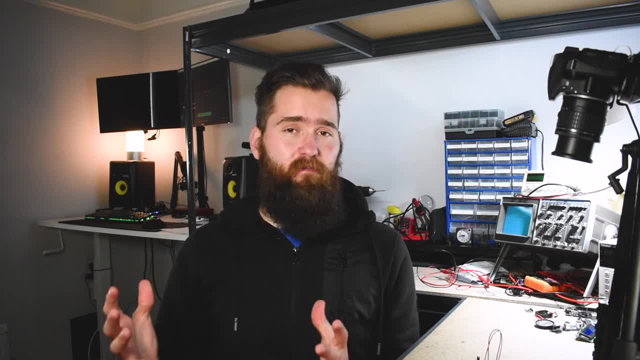 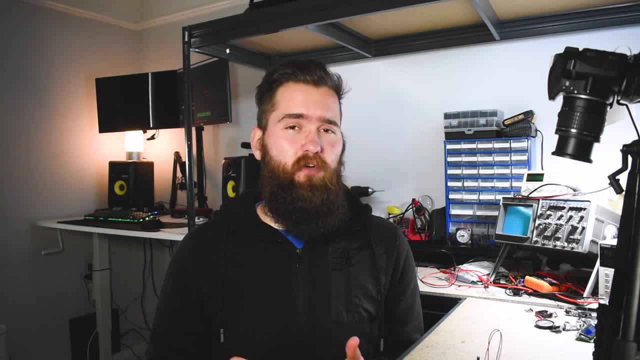 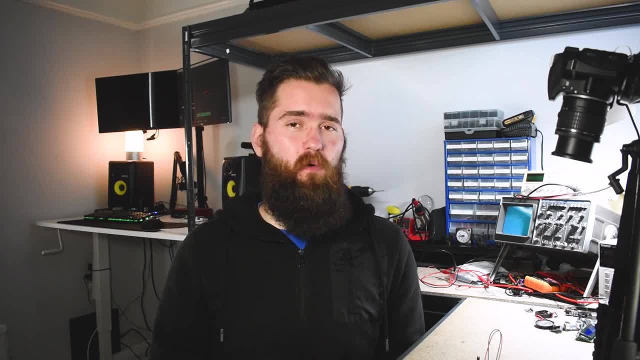 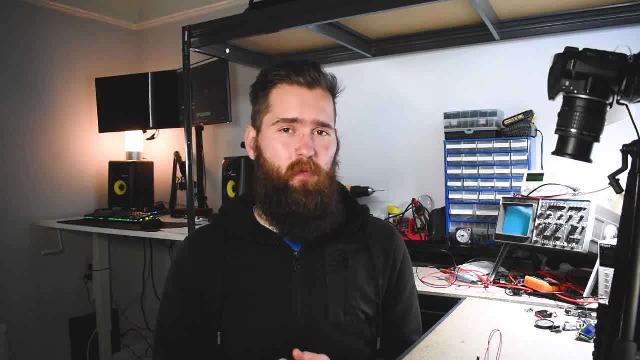 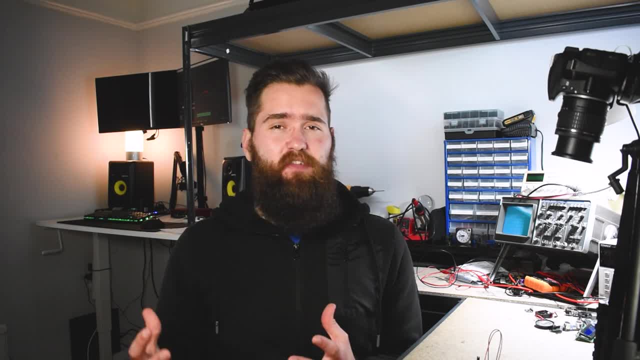 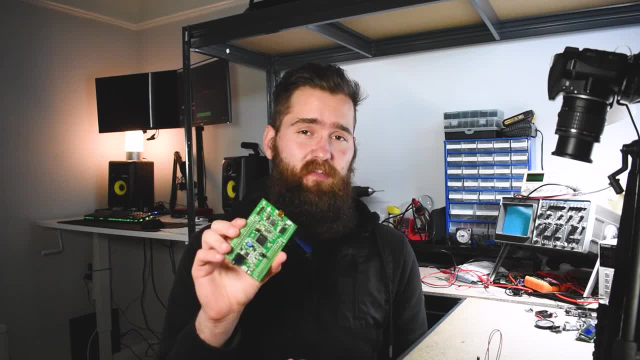 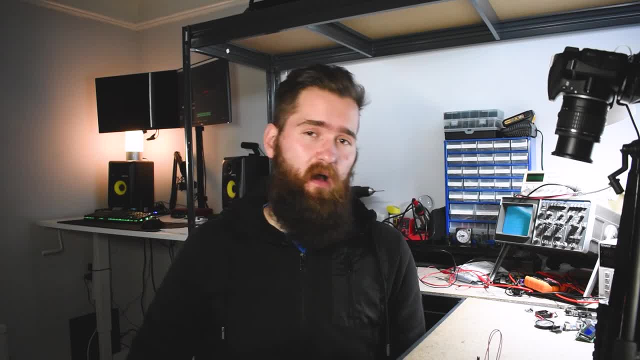 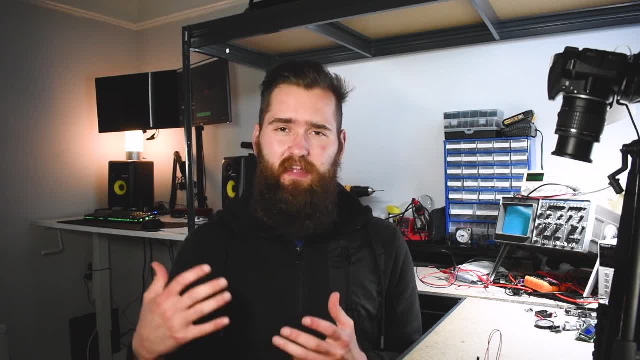 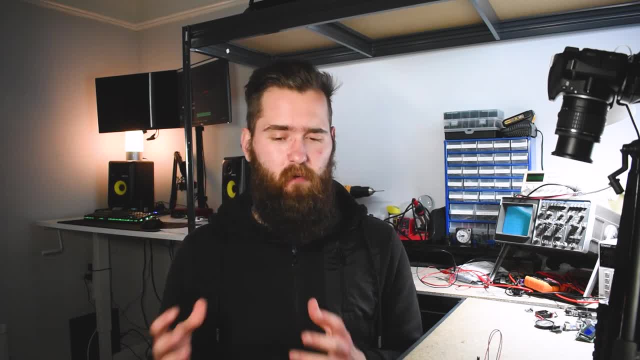 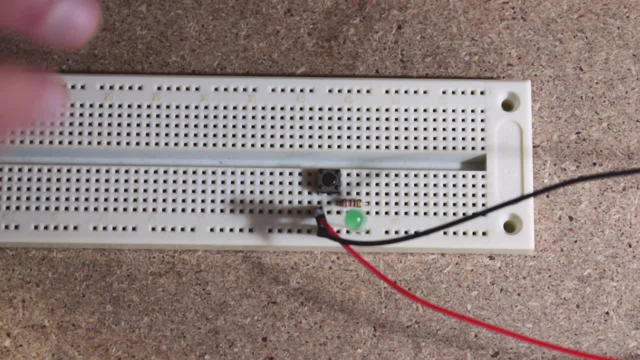 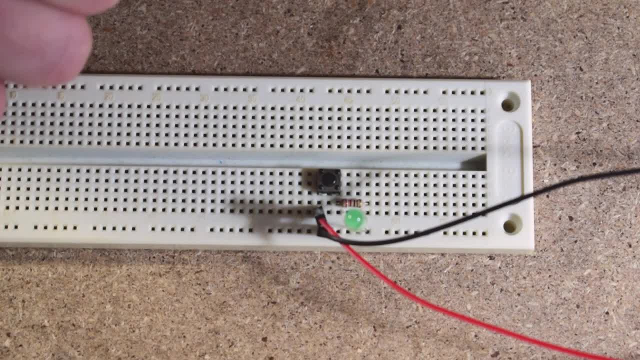 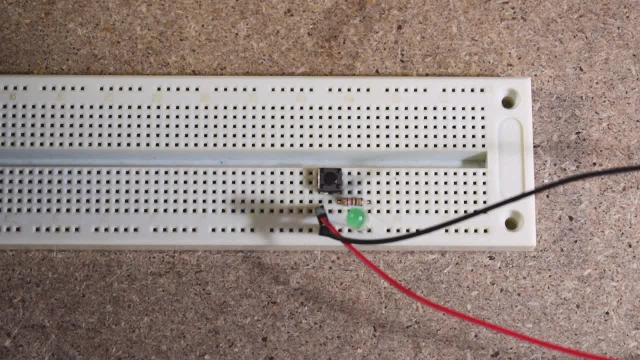 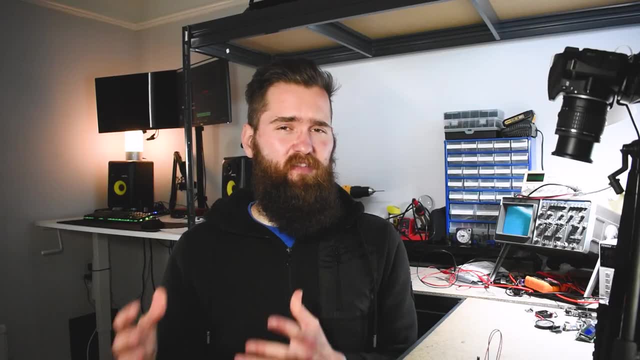 This nuclear board has a larger 100-pin chip, whereas the F4 Discovery board has a larger 100-pin chip. second, I could do this by manually pressing the button every second. While this does work, it isn't very efficient because I'd have to sit here all day and 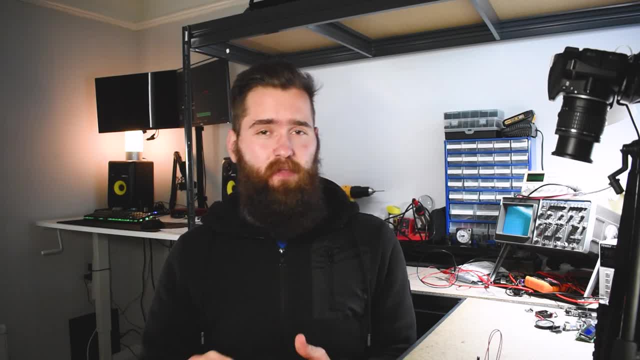 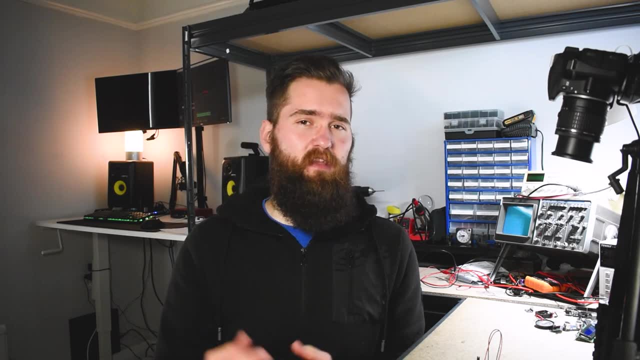 keep pushing this button. Wouldn't it be great if we had something that could flash this LED for us at one second intervals? This is where your micro controller comes in. To tell a microcontroller what it needs to do, you have to write some firmware. Generally, this firmware will be written in. 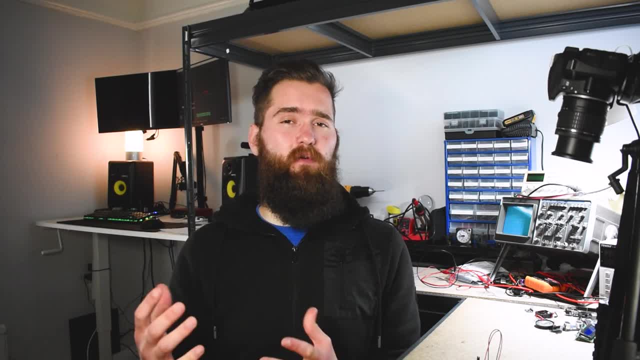 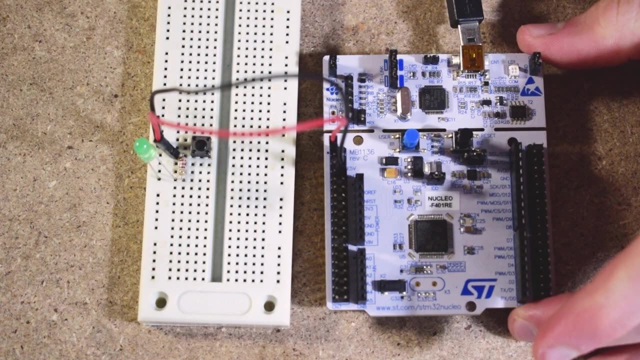 embedded C programming language. After writing the program, we can flash it directly to the memory of the microcontroller and then, whenever we power it up, it'll continuously run that code in a loop. I've written a simple program that toggles this LED on and off every second, As you can see when I plug.